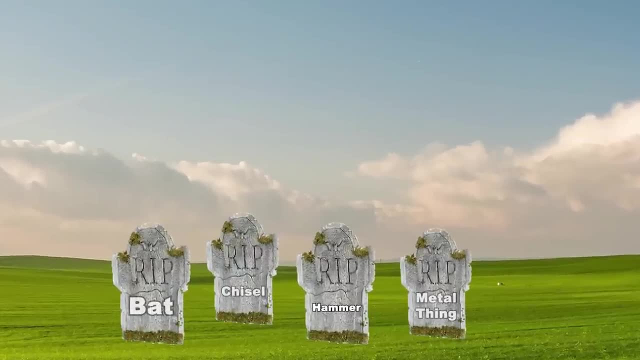 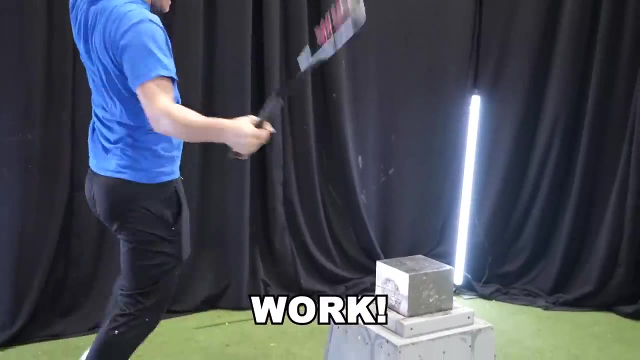 please, Maybe just go ahead and order one more of every weapon, because it's going to be a very expensive video. Home run, Is it? That's not going to work. I had hope. Maybe you break a metal cube with a metal cube. Do your worst. 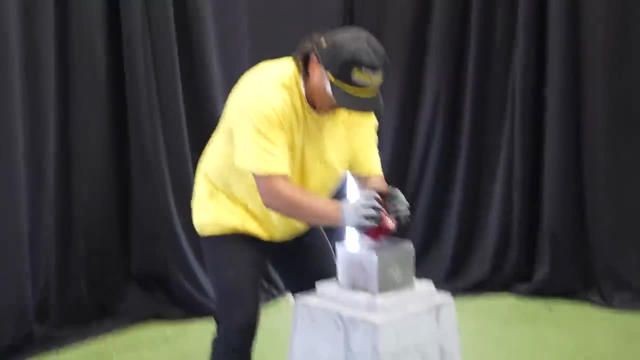 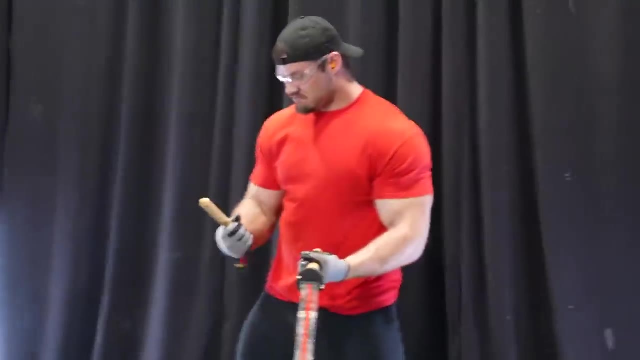 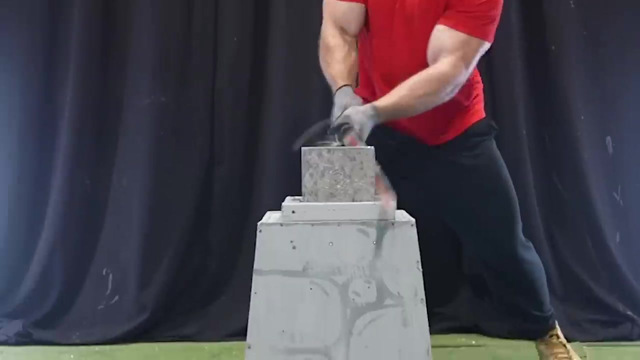 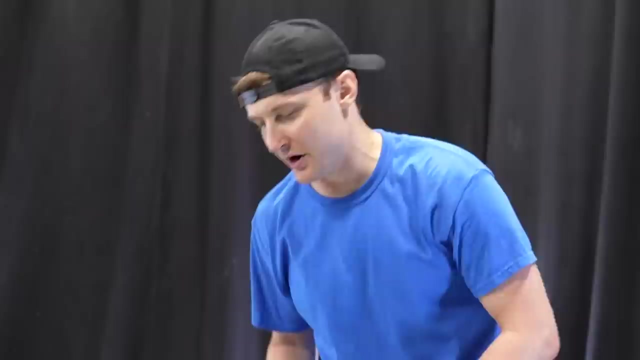 Ah, Whoa Camera idea, Scarlett, come on, It's fine, I'm totally okay with this. Let's go See, this is the key: You get a little slice started and then you put the thing in the slice and then you break. 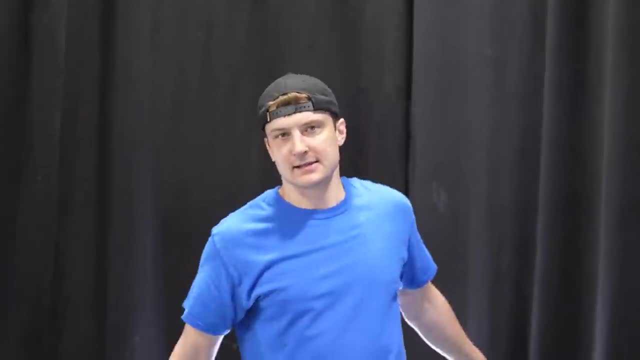 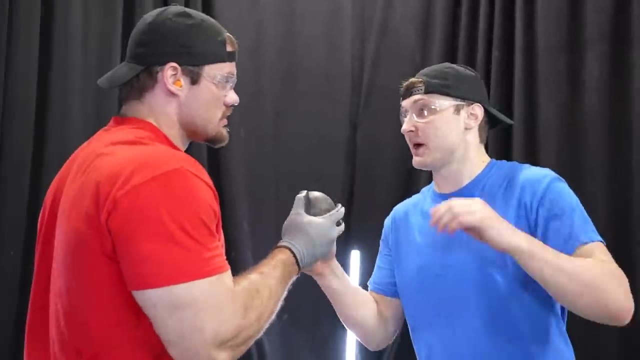 it. Yeah, it's not gonna work. Giant steel ball versus tungsten cube: This is gonna do something. Whoa, I was gonna say be careful, but we're trying to break things, so good job, Never mind, I'm gonna keep my glasses on. 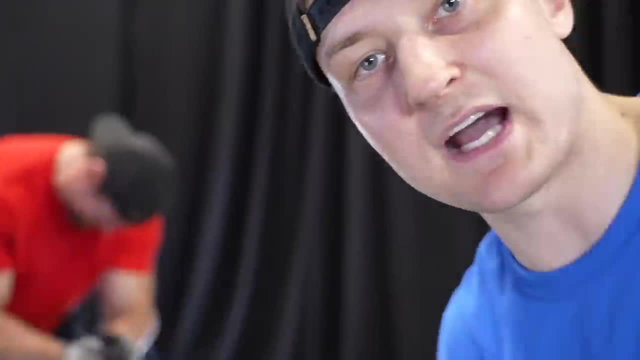 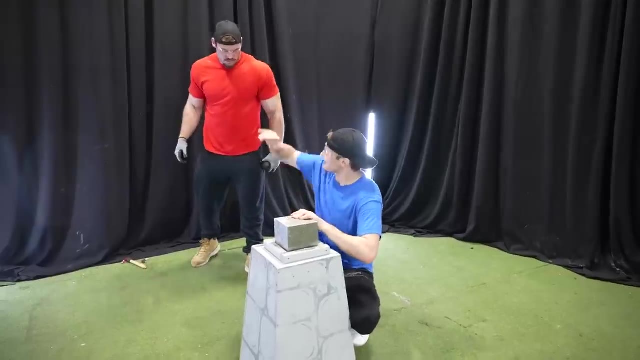 You guys might need some glasses. Here you go. Here you go, Whoa, Whoa. Look at this. Yeah, Let's go Trent, Let's go Trent. Yay, So we got a big. If that was hard, go higher. 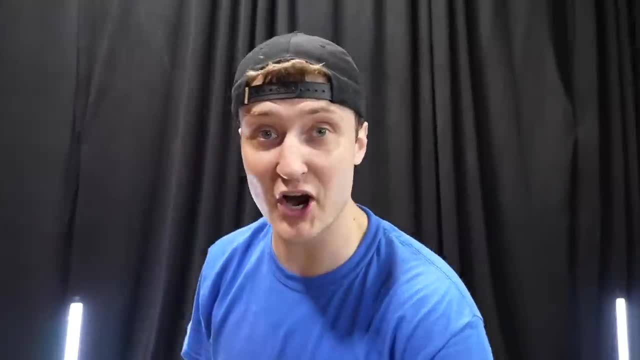 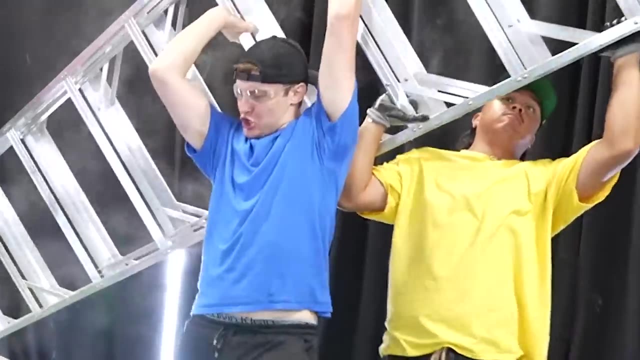 No, This is the biggest ladder we could find. Oh, Oh, Oh, Oh, Oh, Oh Wait, just Did we just throw the ladder at it. Ah, Trent, Trent, here we go. Yo, whoa, whoa, whoa. 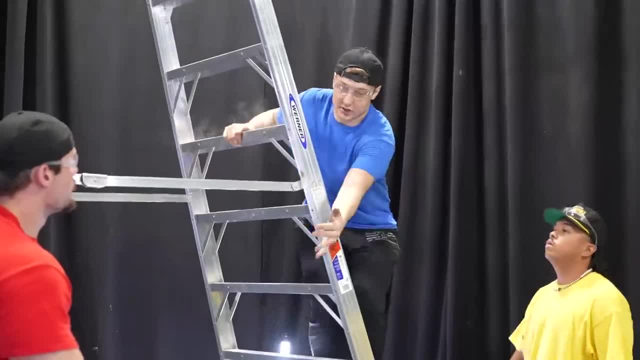 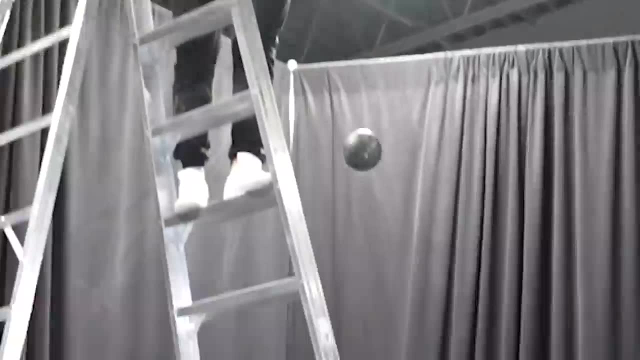 Whoa Hey, Let me just say, it looks way harder from up here. Oh, Again, again, again, again, No damn it, Here we go. Whoa Yeah, Oh, How do you like your tungsten? 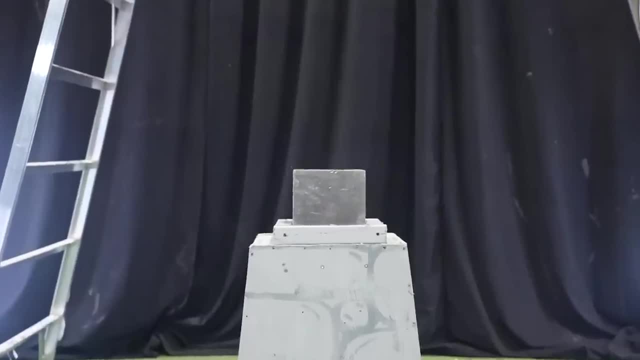 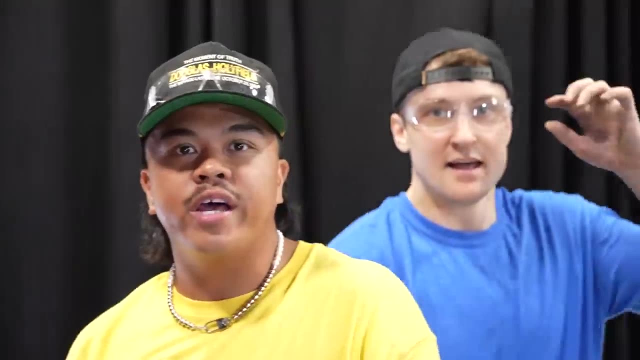 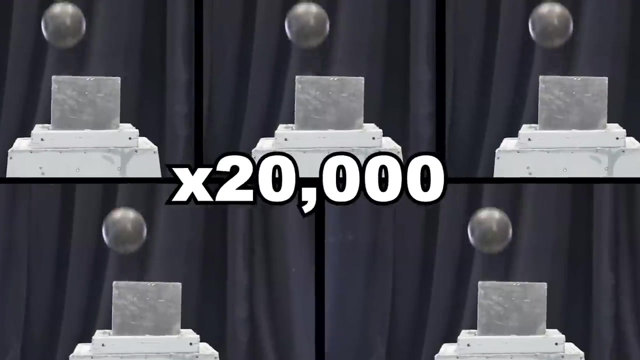 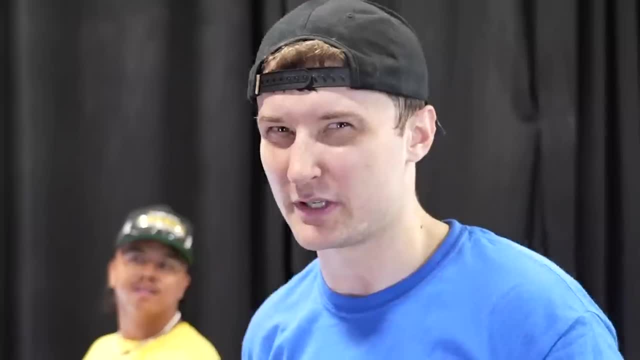 Let's do it. No, no, no. We don't have time for that. 24 hours to break it. We're going to do it. Did I mention Unspeakable? said he'd give us like $25,000 if we broke it. 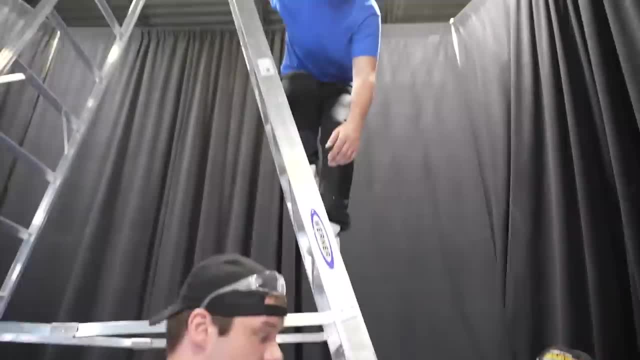 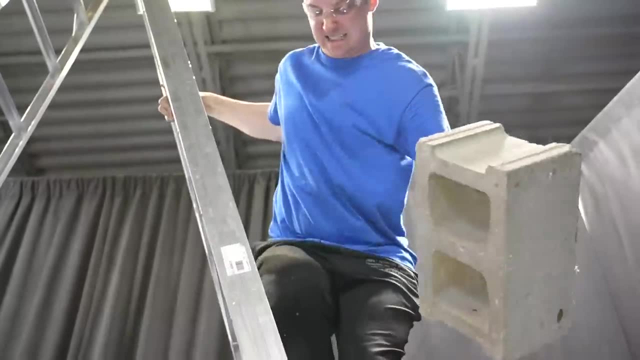 Better go visit an ATM. We were going to drop the cube on a cinder block, but it's too heavy to carry up here, So we're going to drop the cinder block on a cube. Got it? Oh, Did we do it? 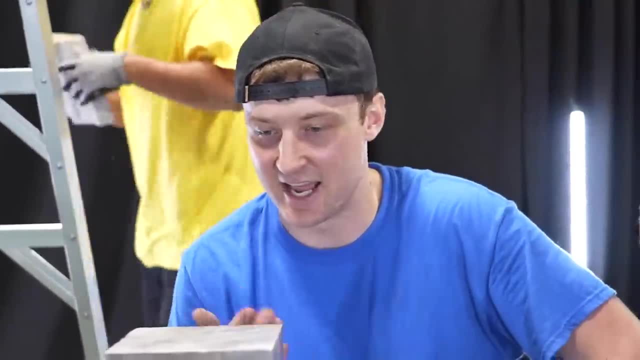 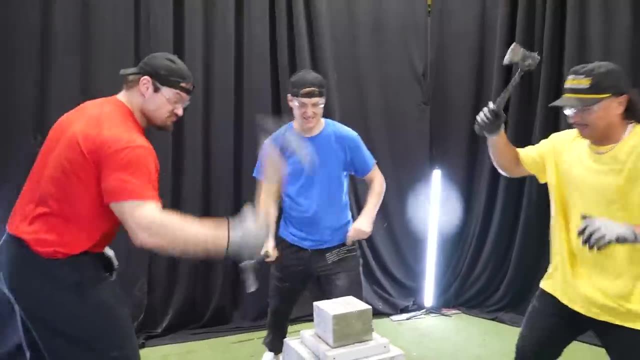 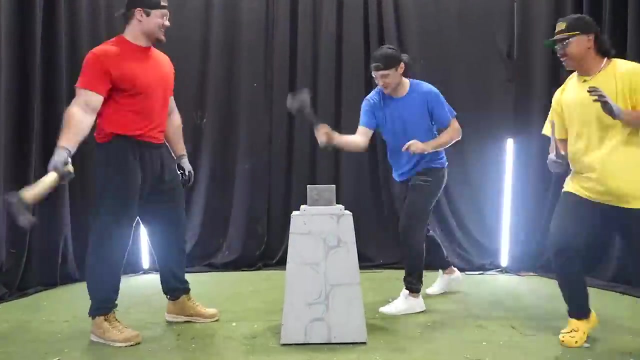 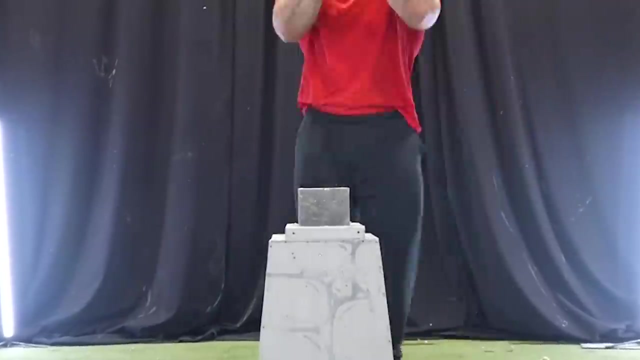 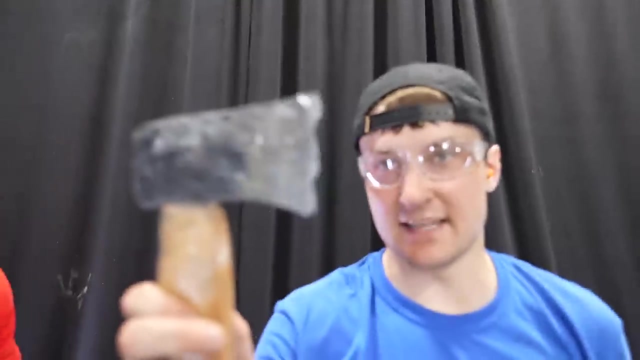 Okay, Nathan, she gave us quite the challenge. Yeah, we need to try something else. access: make a small hole, then we'll make it big. Wow, we're breaking the axis. Let's just, let's just keep going. We've been hitting this and this is what the axes look like. you can have this back now. 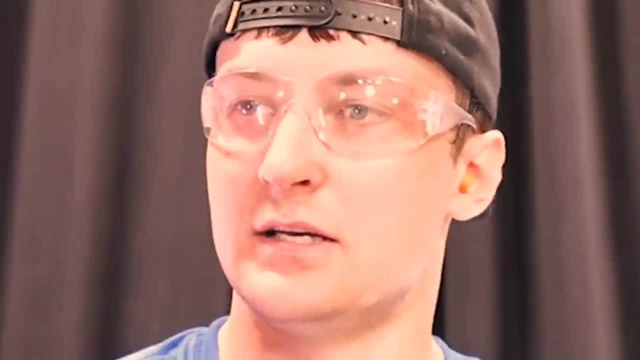 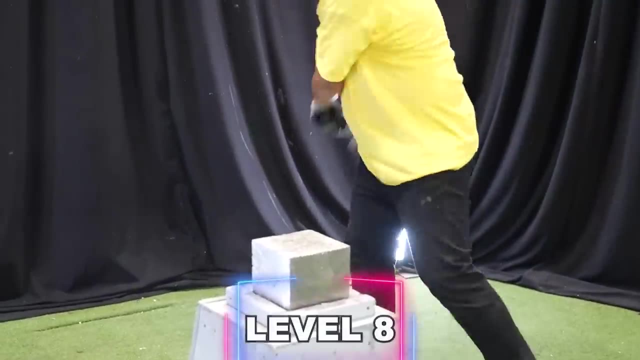 Maybe just keep that, for I try to make an axe out of me, or what. You think that there's damage to the axes? huh? Well, look at this mediocre damage, but still damaged on the left. Oh Y'all, give me gloves, give me gloves. 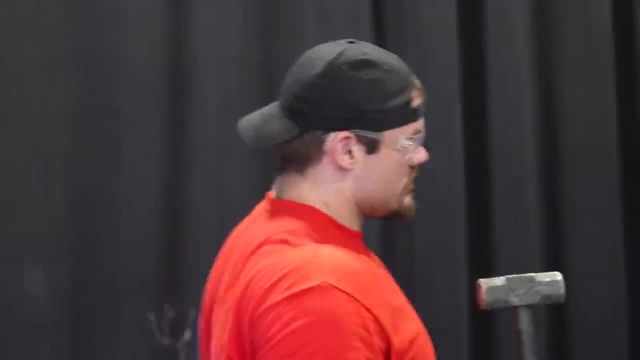 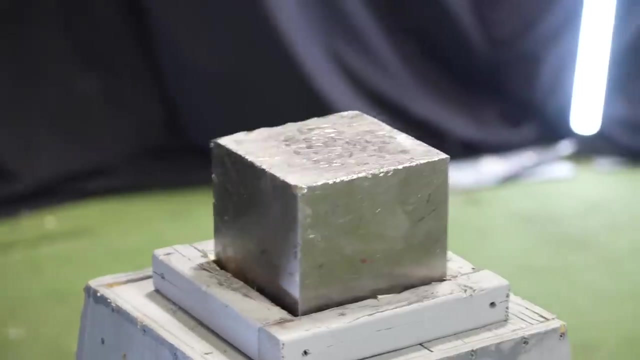 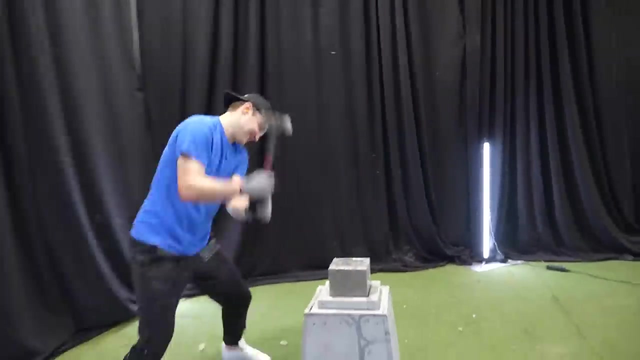 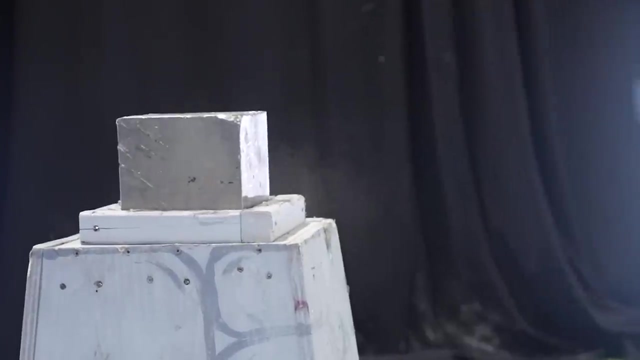 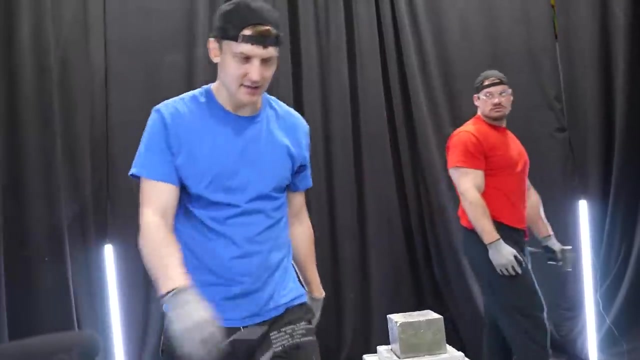 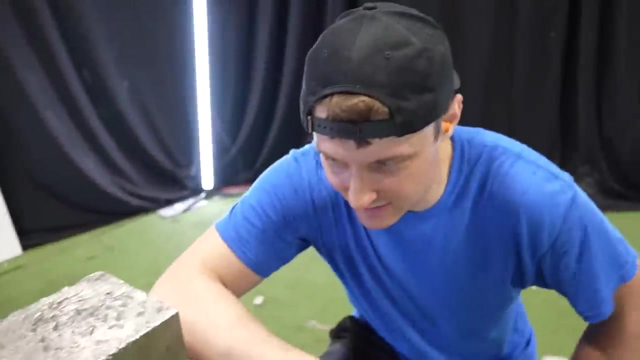 Trent, you got this one dent. I want a dent. Well, I give you Trent. Oh Yeah, let's go. Trent, I want a dent. Come on, we got some damage. It's not a lot In fact, it's just a little speck on the thing. but we also had razor-sharp arrow tips. We don't have those anymore. 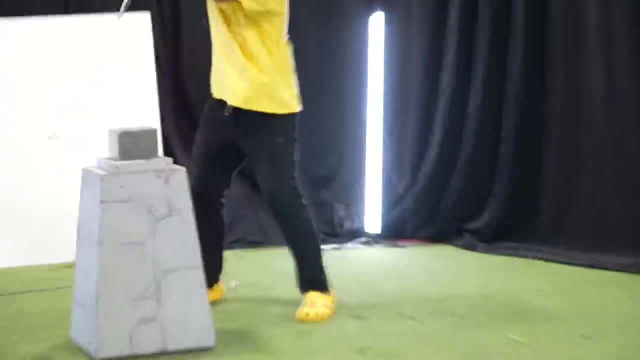 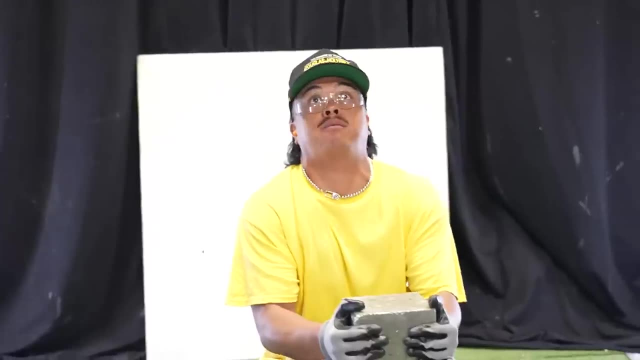 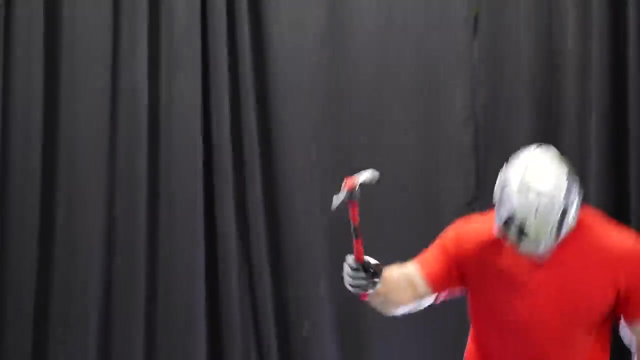 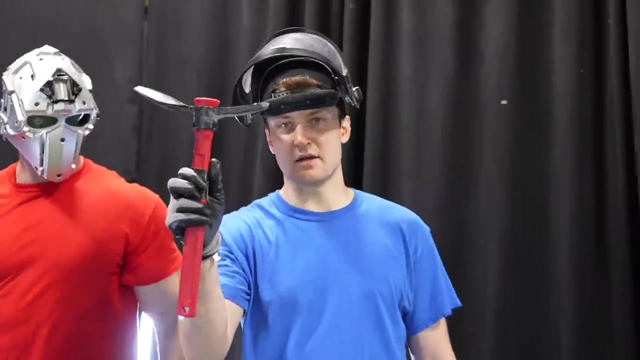 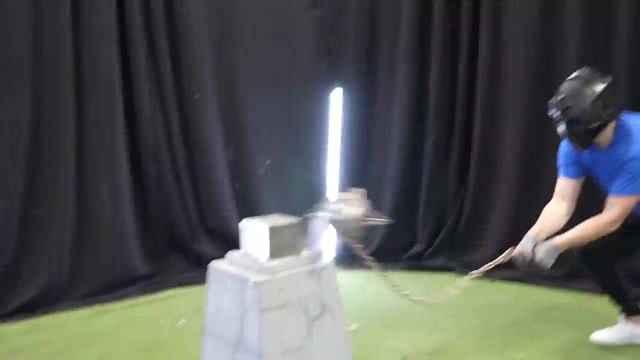 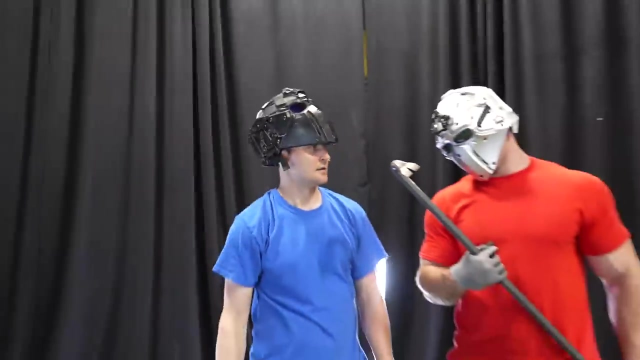 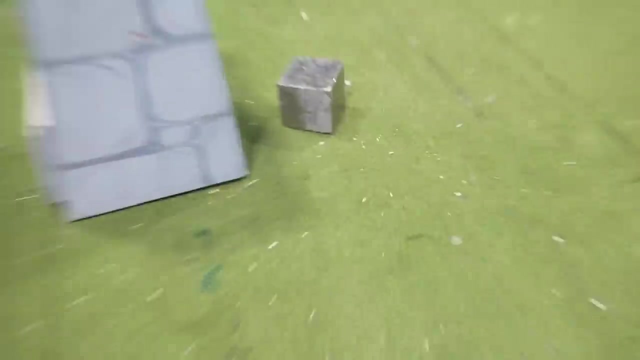 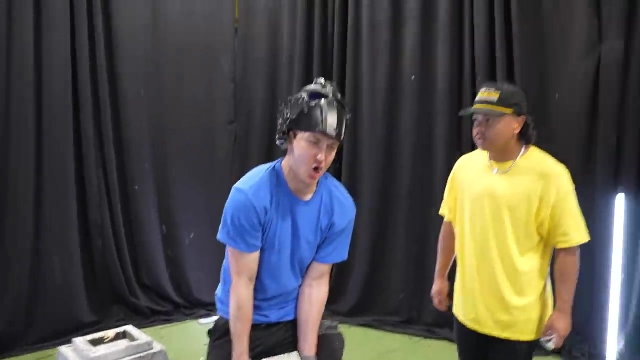 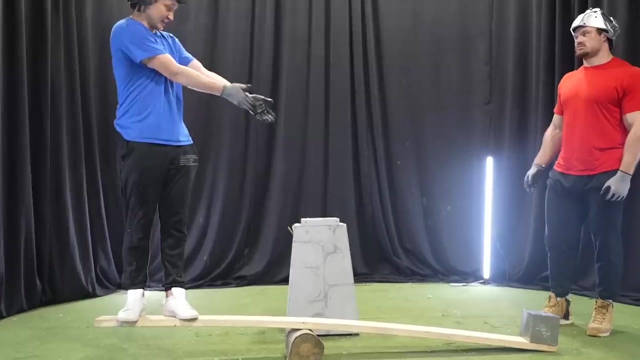 I got this. I like my spear way too much to ruin it. Let's go Trent, This is my pickaxe. now Here we go. I Guess homemade doesn't beat tungsten. They cut my turf. I Weigh 200 pounds. Unspeakable was also giving away $1,000 to anybody who can lift the cube over their head. He didn't have a Trent. 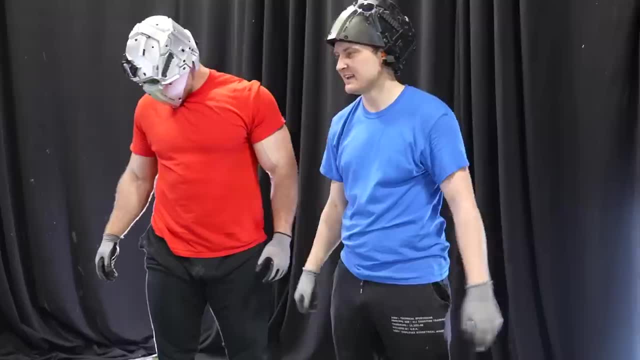 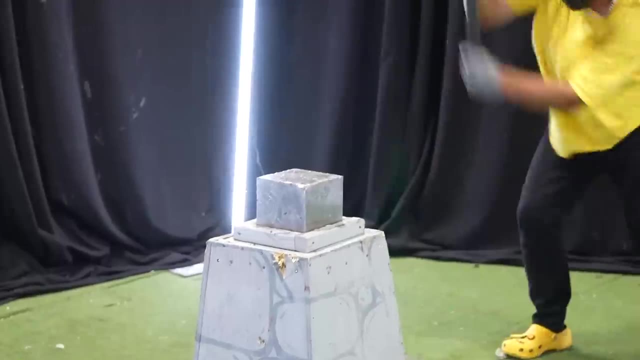 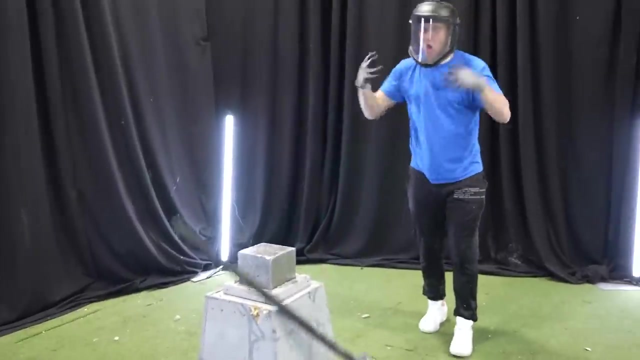 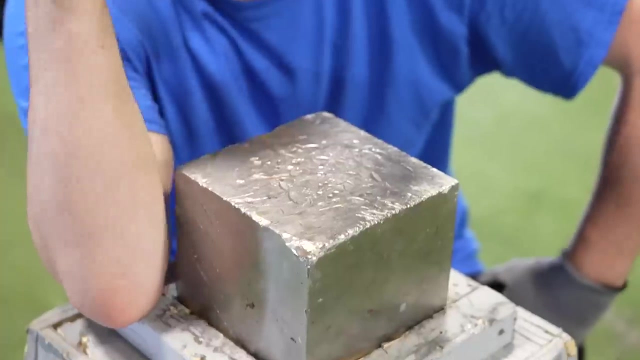 You could have put it there, cuz. now we got to get it, let's go back to breaking it. good job, Let's check the damage. see all this right here. you know what this is. you know we call that. We still need to split it in half, though, Okay. 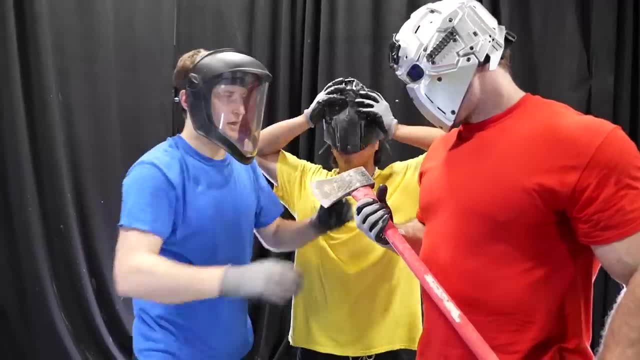 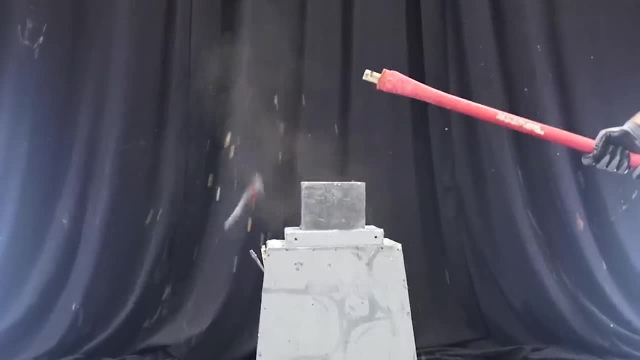 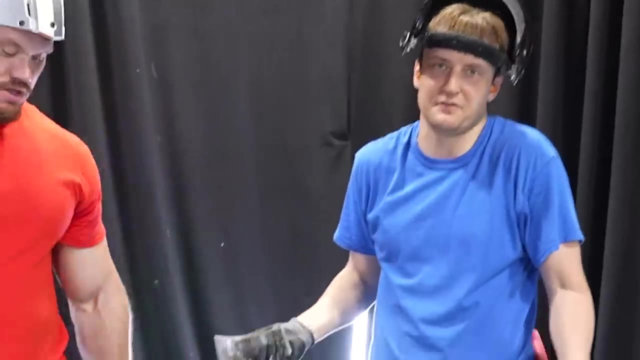 If the small axe taught me anything, What? what just happened? this is, without question, the strongest thing we've ever again gone against ever. This is like The strongest thing on the planet. let's be fair: We're not defeated yet. The only thing harder than tungsten is diamond. Here we go. 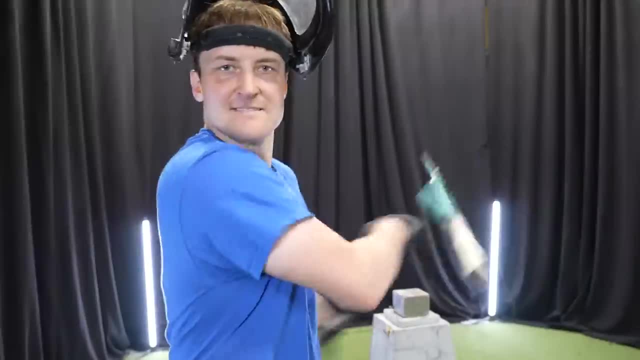 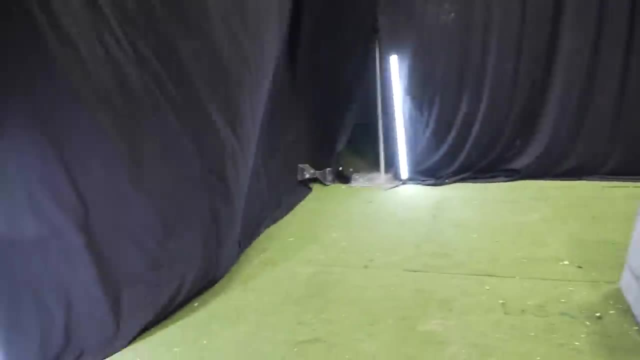 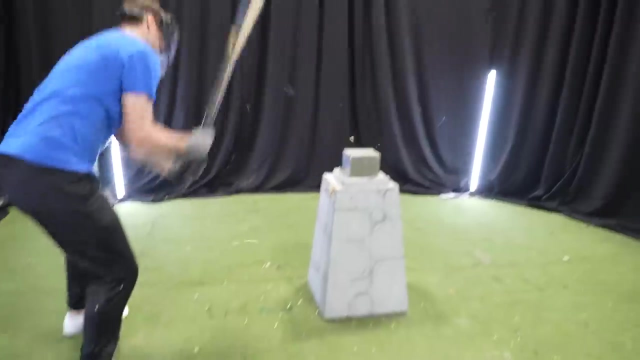 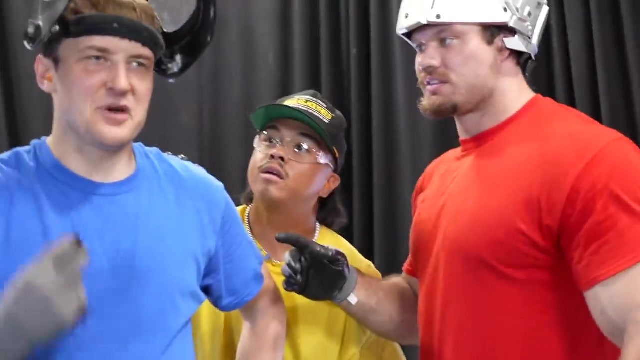 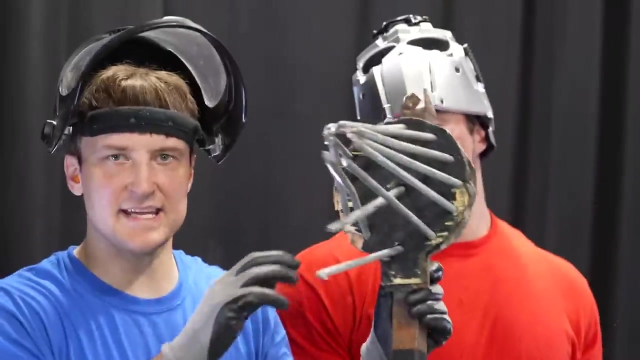 Jeremy, diamond blade is breaking. How does that make sense? What else we got? This shouldn't be a club Guys little club who pays for these weapons. I did: Okay, we need to break this to get some money to buy new weapons. Spike has literally broken everything and now spike is broken. I don't know if I want to continue, because I don't want to break. 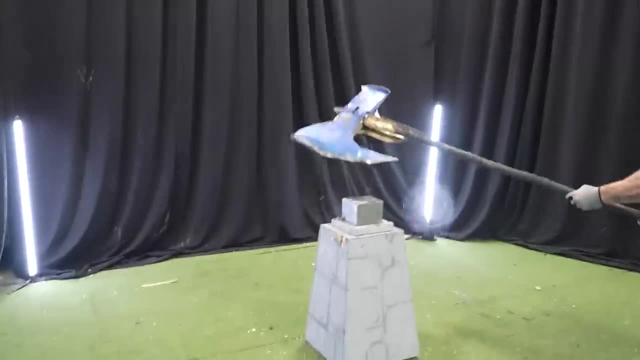 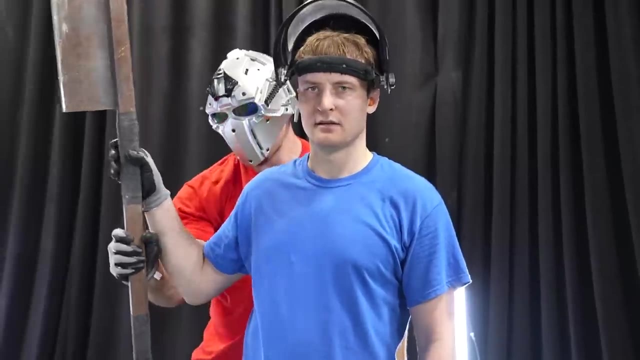 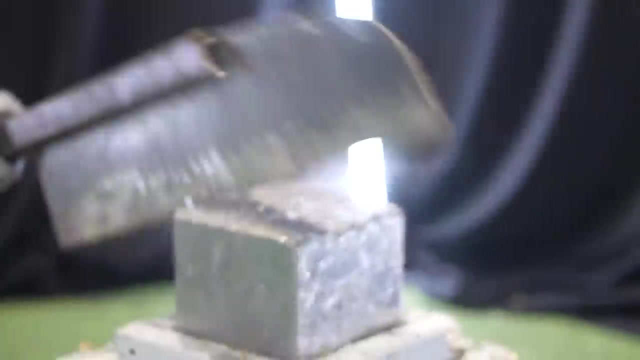 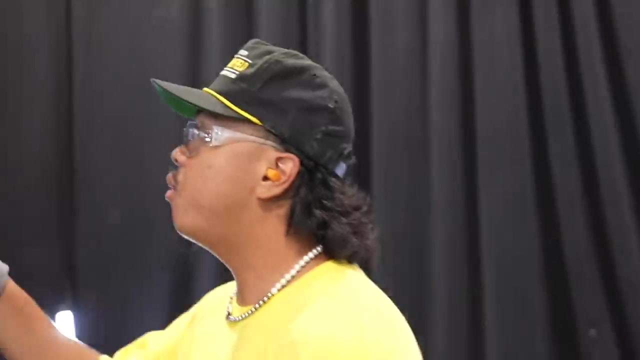 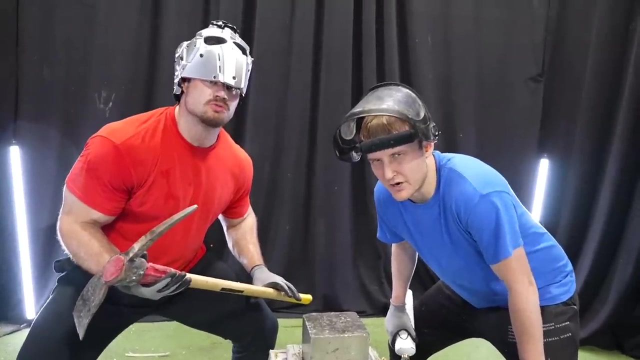 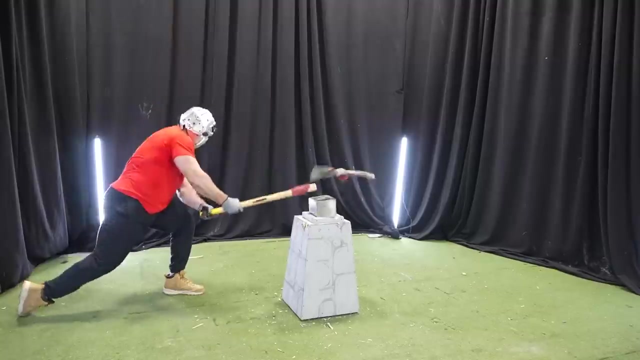 anything else. I got another thing for you to break leadership. Okay, anything, But for the next day ahead, Take care. See you next time. I don't have to do. I don't know either. We've been working real hard, but now it's time to work smart. We got a pickaxe and we got a blowtorch. Oh, what Needs to break it again? We are oppressors here. hasta steak is wrecking Sabanis, we are rock and ready. we got to blow our chance- no problem, This one about the soupUp- and will do until never know what to use next. Let's go first and don't panic. Okay, Monday is my1 last day for tonight'se reason. nobody is uncertain schedules, FYI, we'll be right back after Monday. See you on Wednesday, okay, Bye. 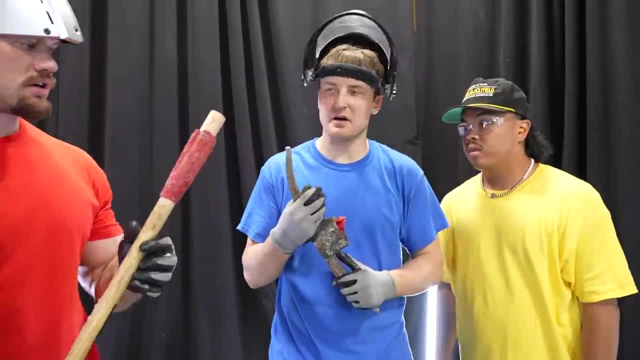 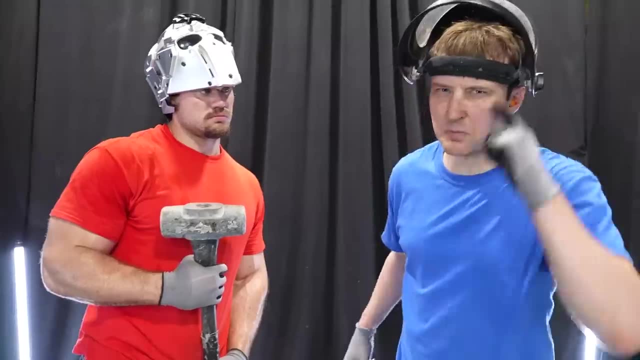 survived every video we've done ever. I'm actually sad about this- me too, Nathan. let's have a dark side, but you're not gonna win. I got something thinking: smart. co2 makes metal cold. we're gonna make it cold. he's gonna hit it here we.